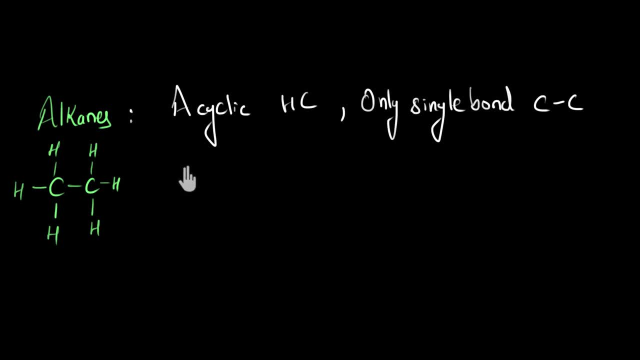 All the carbon atoms will be connected with a single bond. No double or triple bond will be present between them. So probably the simplest alkane is going to be one with one single carbon, One single carbon, Methane- And this carbon is going to have four valence electrons which it will be sharing with. 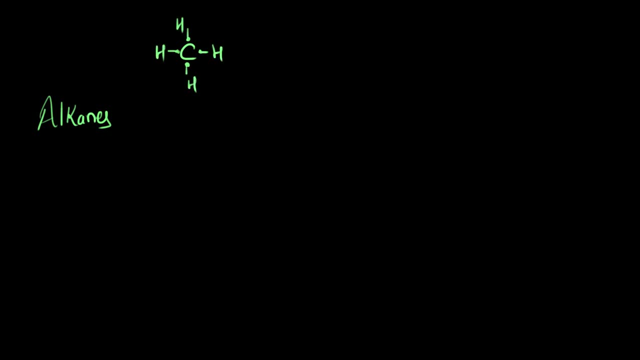 four hydrogen atoms to fulfill its octet and be stable. So this is the first member of the alkane family. But that's not it. I can keep on replacing a hydrogen atom with another carbon atom and keep on elongating this chain. Something like this: Here I replace a hydrogen atom with 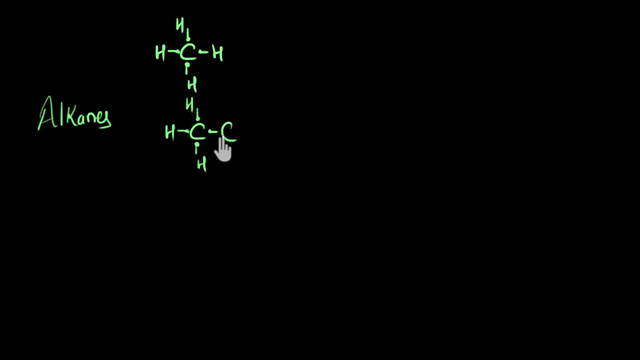 another carbon atom. So see, here this carbon is sharing one electron with this carbon And it will be sharing the rest of the three electrons with hydrogen atoms. So this is also a valid member of the alkane family. See, this is acyclic And all the carbon. 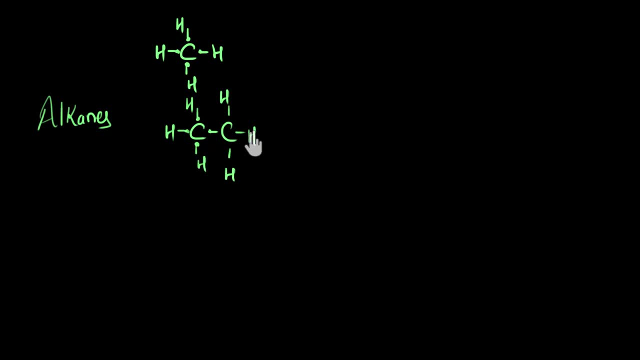 atoms have single bonds with each other. There are no double or triple bonds in this compound, right? So this is another alkane. Now, similarly, I can keep on elongating this chain. I can take a copy of this compound and replace a hydrogen with another carbon. 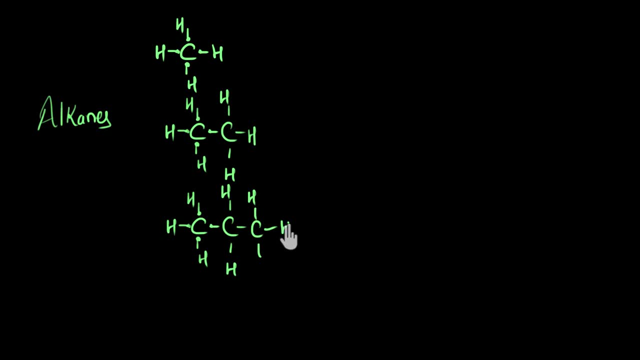 And fulfill its valences with hydrogens. So this is another member of the alkane family. There are three carbon atoms in this particular chain. I can keep on doing this again. This has four carbon atoms, So you can imagine that similarly, I can keep on forming newer and. 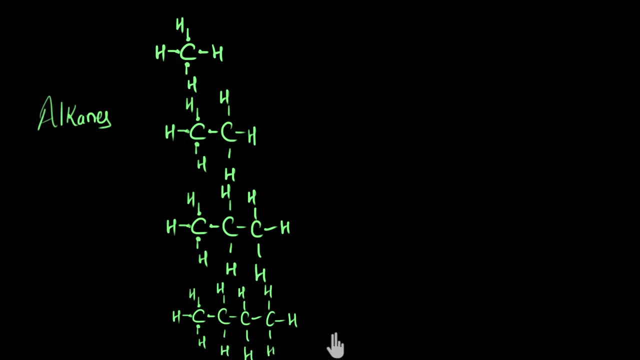 newer alkane members. I can have five carbon chain or 10 carbon chain or 20 carbon chain. So here we saw how to find out the members of the alkane family. Now let's try to find out their general members. So let's start with the alkane family. So let's start with the alkane family. 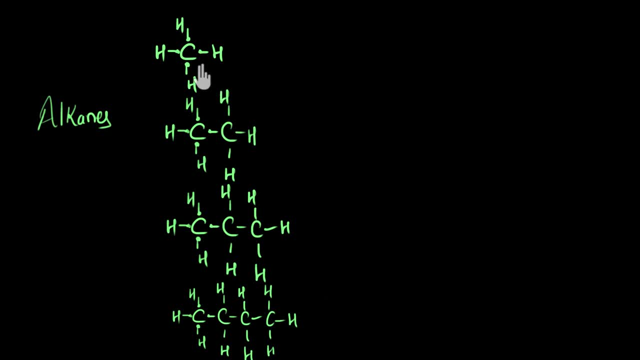 molecular formula For this. let's try to write down the molecular formula for each of these compounds. So methane here has one carbon and one, two, three, four, four hydrogens. So its formula is going to be C1C and H4 because there are four hydrogen atoms. Similarly, this compound, this has 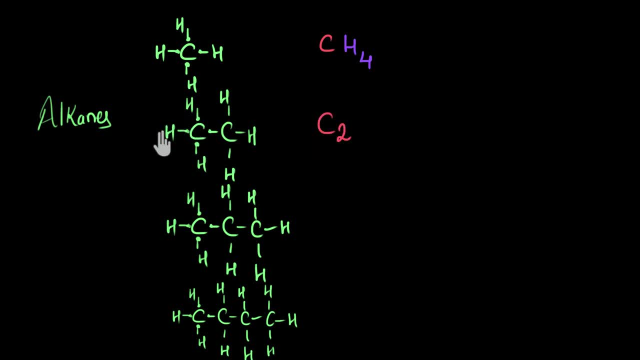 two carbon atoms, So C2, and there are one, two, three, four, five, six, six hydrogen atoms, So C2H6.. Similarly, can you pause the video and try to find out the members of the alkane family? So let's. 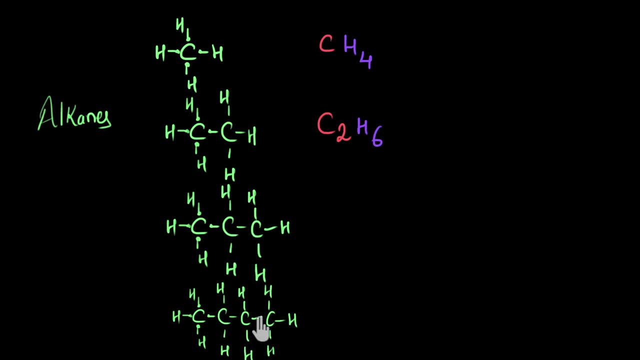 try to find out the molecular formula of these two molecules. Now that you have tried it, let's see. So this one has three carbon atoms, So C3, and it has three, four, five, six, seven, eight, eight hydrogen atoms, So C3H8.. Similarly, this one has four carbon atoms, So C4, and it has three. two, five, six, seven, eight, nine, 10, 10 hydrogen atoms. Oops, let me change the color. C4H10.. This is going to be its molecular formula. Now let's see what is the general molecular formula of alkane family meaning. what is the common? 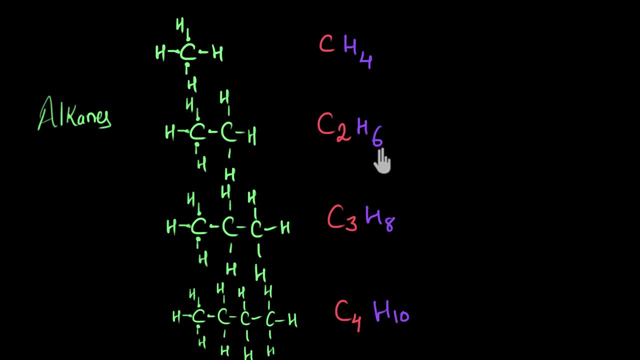 relationship between the number of carbon atoms and the hydrogen atoms in every alkane. So basically, what we are trying to find out is if, given an alkane which has N carbon atoms, can we somehow tell how many hydrogen atoms are going to be present in this alkane. Okay, So let's see. So over here I see that for two carbon atoms. 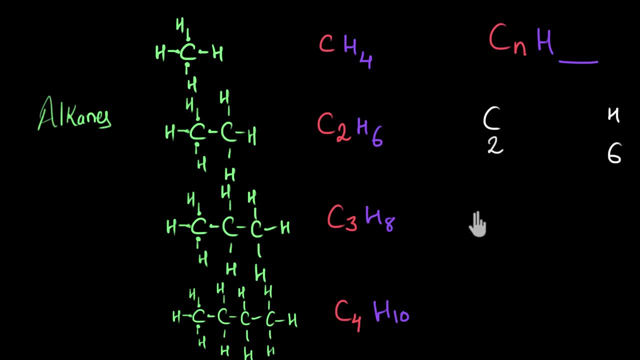 there are six hydrogen atoms. Here for three there are eight, Here for four. carbon: there are 10 hydrogen atoms. Hmm, What is the relationship between the numbers of carbon and hydrogen atoms? If you can find that, we can arrive at a general molecular formula, So can you pause the video over here and 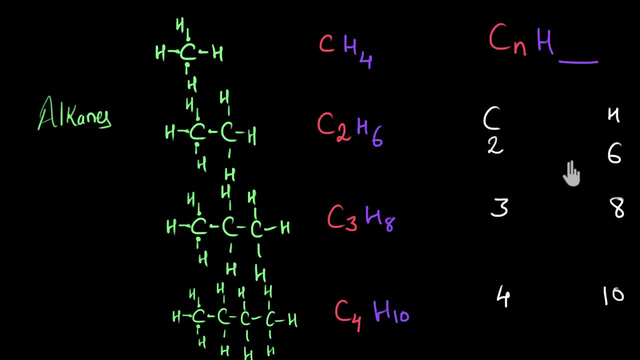 try to figure out the relationship between these two numbers. Pause and try by yourself first. Now, if you have tried it, let's see. So here, maybe if I multiply two with three, then I get six, So maybe into three is the relationship. Let's try. 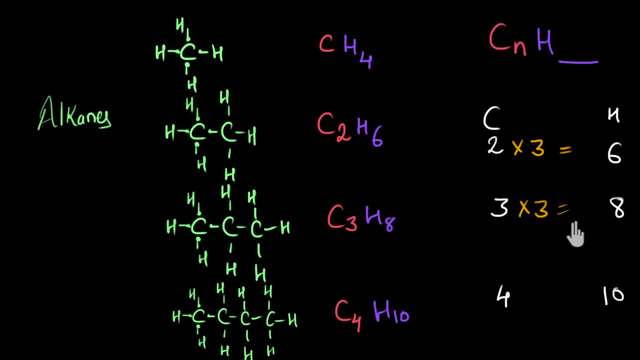 that out, Three into three, this is going to be giving me nine and not eight. So multiplying by three is not the right relationship. How about addition? Maybe if I add four over here, four plus two, six. Okay, Let's add four over here. No, I'm not getting eight over here, right? So adding four. 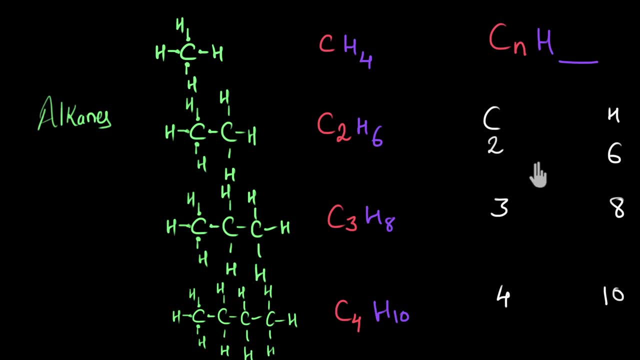 is also not going to be the relationship. How about I do both, I multiply, and then I add some number, Like, for example: I multiply two with two. Two twos are four plus two. Okay, Then I am getting six. Let's try the same over here: Three into two. 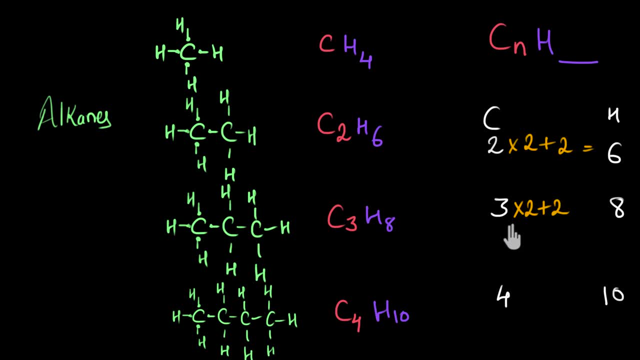 and plus two. Maybe this is the relationship Into two and plus two. So three twos are six plus two is eight. Oh wow, I'm getting this number Again. let's try it one more time. Into two and plus two: Four twos are eight plus two is 10.. So yes, this is the relationship. 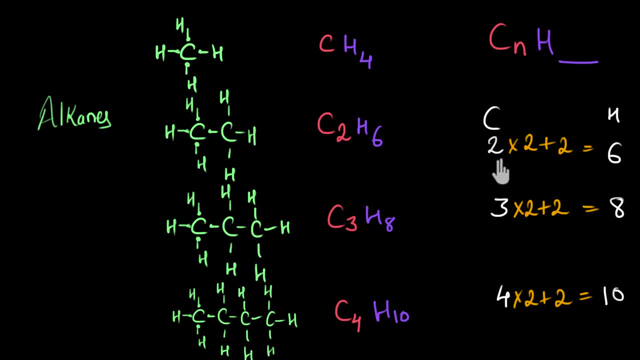 for alkane family. Now, if you take the carbon atom and multiply it by two and add two to it, then you will get the number of hydrogen atoms. Okay, So over here our general formula is going to be: if the number of carbon atoms are N, then I'm going to multiply this by two. first, 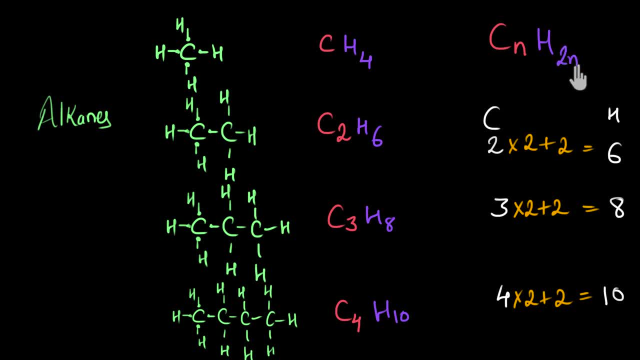 So that'll give me two N, and then I'm going to add two to it. This will be the number of hydrogen atoms present. So this is the general molecular formula for the alkane family, All the alkanes according to this ratio. only. If tomorrow you come across any alkane which has, let's say, 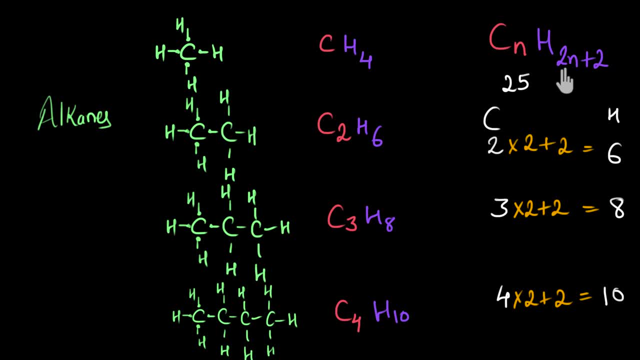 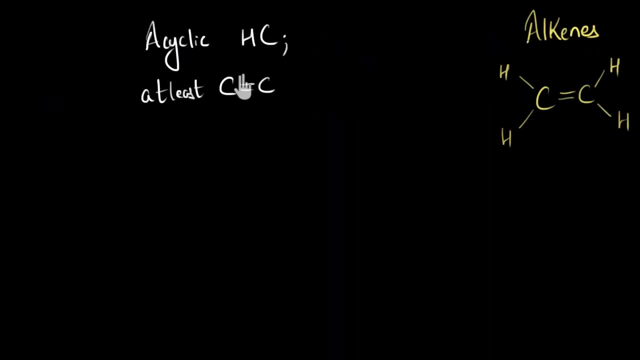 25 carbons, then the number of hydrogens will be twice of 25,, which is 50, plus two 52. So C25H52 will be the molecular formula. Isn't that very convenient. Now let's move on to alkenes. So alkenes also are acyclic hydrocarbons. 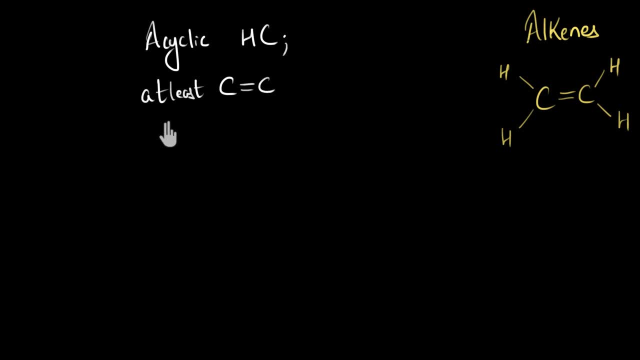 meaning the carbon atoms are not arranged in a circular pattern And they have at least one pair of carbon atoms with double bond between them. Okay, There can be more, but at least one pair of carbon atoms, and this is an example of alkene. Now can you pause the video and think about? 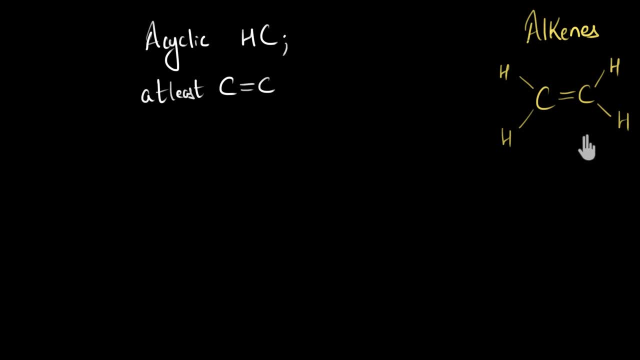 whether there can be an alkene with just one single carbon atom. Pause and think So no right, That's not possible, Because we know that alkene need at least one pair carbon atoms with a double bond in between them. So on pair means at least we need two carbons, right? So an alkene with a single carbon atom is not possible. just to think that these two would be the same things that you would do If you are always using carbonon perceived. 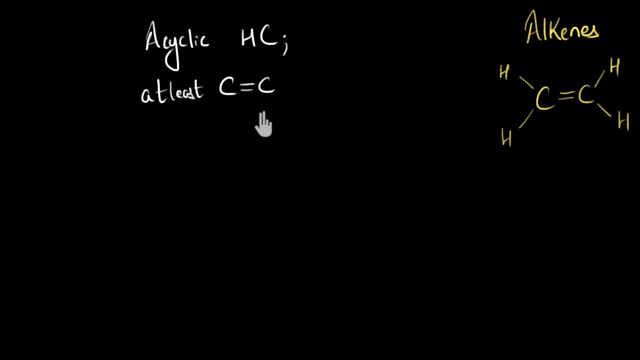 So one pair means at least we need two carbons, Right? So an alkene with a single carbon atom is not possible. So no one carbon atom can be future. In that case the carbon atom is potential, Thank you. so an alkene with a single carbon atom is not possible. so here i have two carbons with a double. 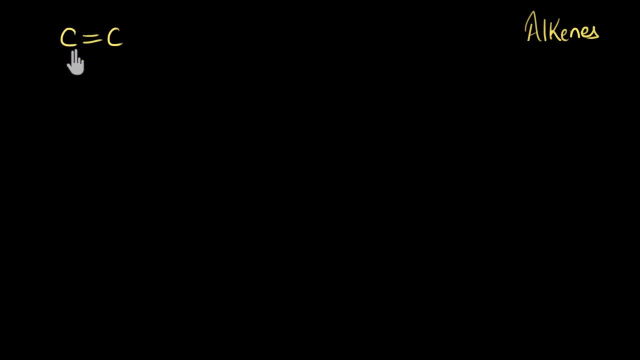 bond in between them. okay, now that this carbon is sharing two electrons with this carbon, there are two more valencies, two more electrons pending. right, these will be satisfied by hydrogen, hydrogen. similarly over here, hydrogen and hydrogen. okay, now, this is just the first member, just like how in? 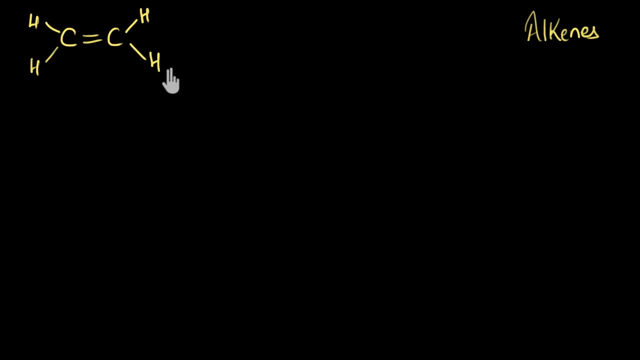 alkanes. we took a copy of the first alkane and we replaced hydrogen with more and more carbon atoms and elongated the chain. we can do similar things over here also. let's do that now. this carbon is sharing one electron. with this carbon, now the three. 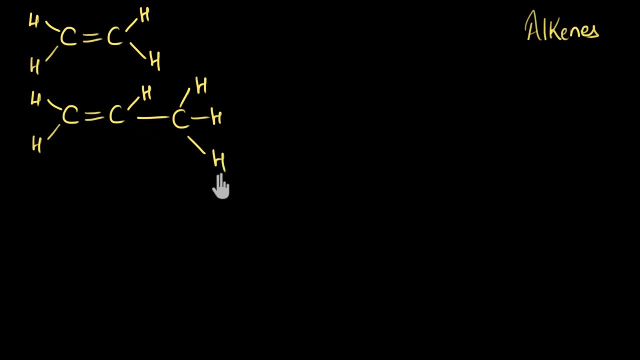 pending electrons will be shared with hydrogen atoms, so this is another member of the alkene family. see, this is acyclic in nature and it has got one pair of carbon atom with a double bond in between them. See, there can be more than one, okay. 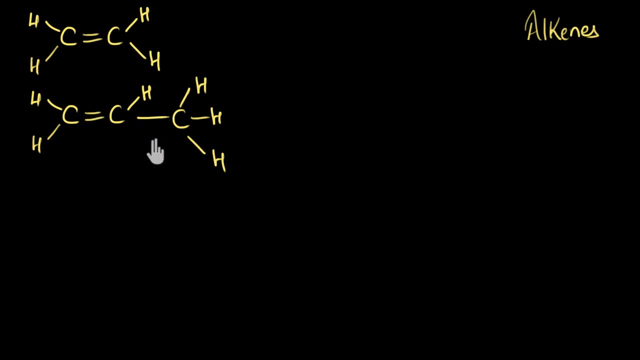 There can be a double bond over here also between these two carbon, But in this video we are talking about simple alkenes, meaning alkenes which have only one pair of carbon atom with a double bond in between them, And we will be trying to write. 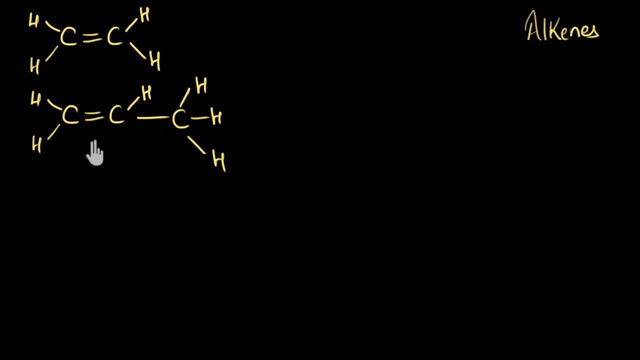 the general molecular formula of simple alkenes. okay, Now, before doing that, let's write the next member of this family. Let's take a copy of this and let's replace the hydrogen atom with another carbon. So this is another member of the simple alkene family. okay, 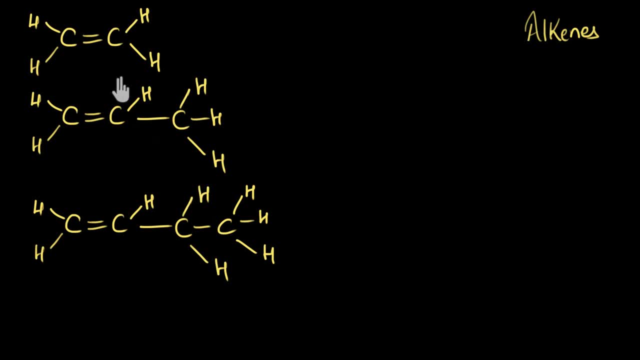 Now let's try to find out their molecular formulas. So over here I can see that there are two carbons, so C2, and then there are four hydrogens, so C2H4.. This will be its molecular formula. This has three carbons, so C3,. 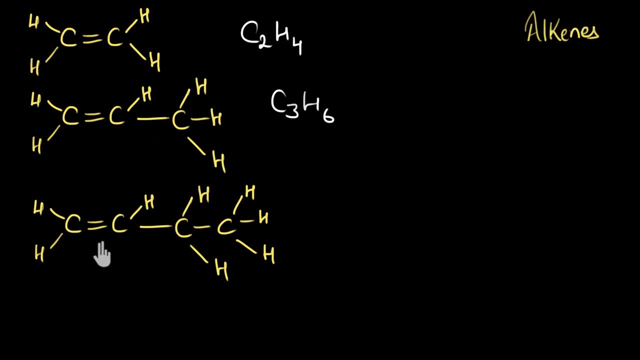 and one, two, three, four, five, six, six hydrogens. This has one, two, three, four carbons C4, one, two, three, four, five, six, seven, eight, eight hydrogens. 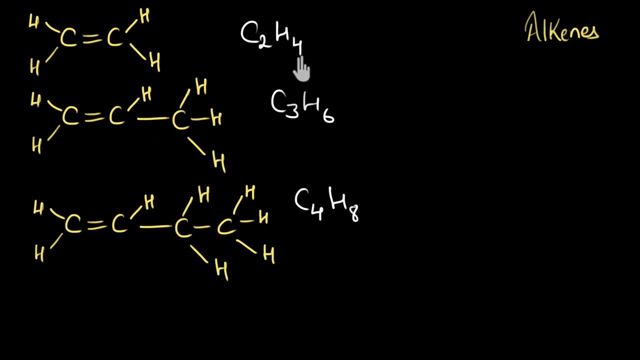 So over here you can clearly see that the number of hydrogen atoms they are double the number of carbon atoms. See over here: four, two, six, three, eight and four. That means the general molecular formula can be Cn. 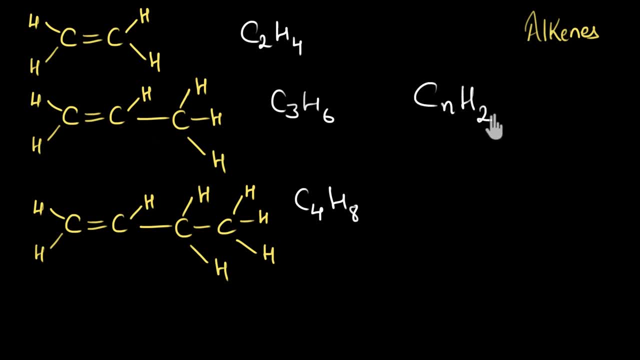 If there are n carbons, then the number of hydrogens have to be twice the number, twice the number 2n. So this is the general molecular formula of alkenes. Now let's talk about alkynes. See, alkynes are also acyclic hydrocarbons. but they have at least one pair of carbon atoms with a triple bond in between them. a triple bond okay. And for similar reasons, like alkenes, we cannot have an alkyne with just one carbon atom. We will at least need two carbon atoms. 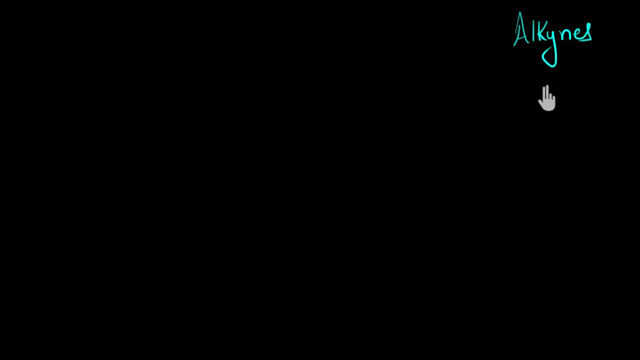 with a triple bond in between them. So the simplest alkyne will have at least two carbons in it. Okay, Two carbons and there will be a triple bond between them. Okay Now, since this carbon is sharing its three electrons. 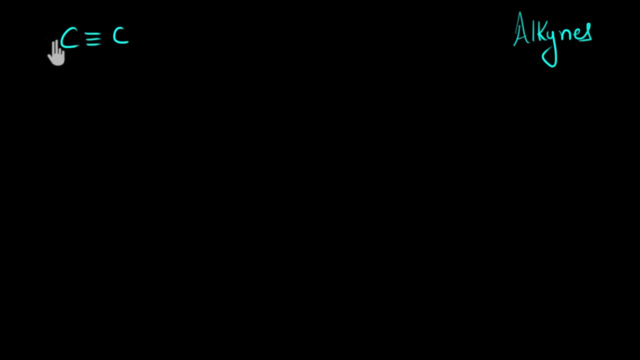 with this carbon. it has one more electron left in its valence shell which it will share with hydrogen atom. Similarly, this will share with hydrogen atom. So this is ethane. This is your simplest alkyne. And now, just like how we did in case of alkenes and alkenes, 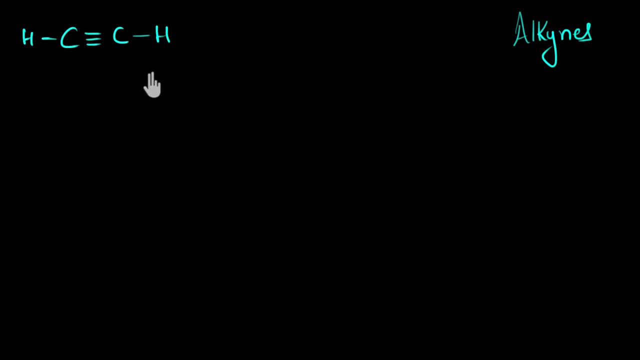 here also, we can increase this. we can elongate this carbon chain and form many other members of the alkyne family by replacing hydrogen with more and more carbon atoms. So let's do that, If we copy paste and replace this hydrogen with a carbon atom. 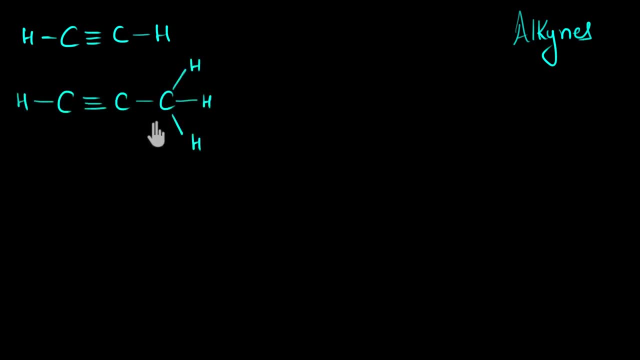 then we will get something like this. So here we have a chain of three carbon atoms, and one pair of carbon atoms have a triple bond between them. So this is also a simple alkyne. Now let's elongate the chain by replacing this hydrogen. 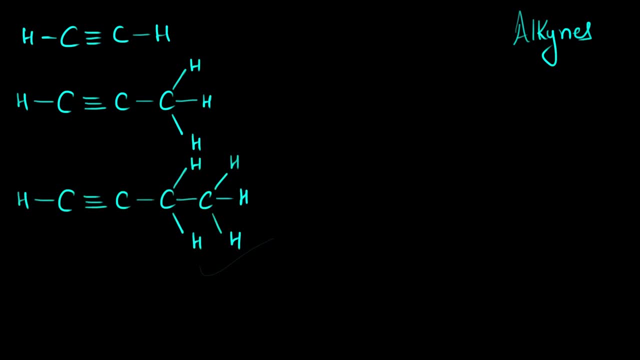 with another carbon. Then we will get something like this: Here we have a chain of four carbon atoms and one pair of carbon atoms have a double, have a triple bond in between them. So this is also a simple alkyne See over here we can have more than one pair of carbon atoms. 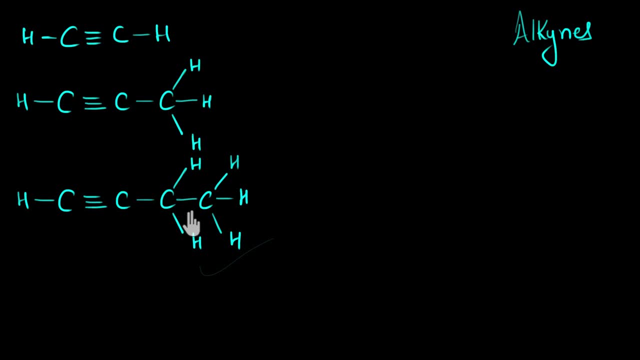 with triple bond, Like we can have a triple bond over here also. But see, those are complex structures In this video. we are not talking about them Here. we are only talking about simple alkynes, meaning alkynes which have only one pair of carbon atoms. 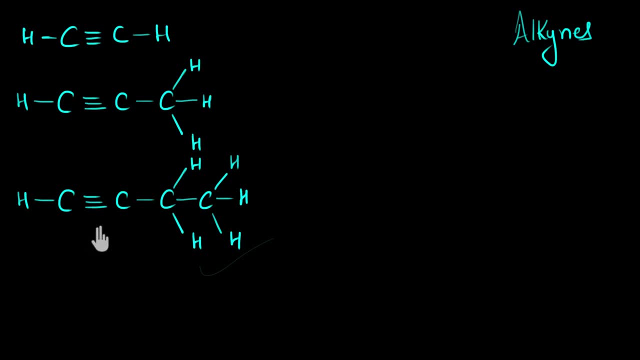 with a triple bond in between them. Now let's try to figure out the general molecular formula of simple alkynes. Now, before I do that, can you pause the video and try it by yourself? Basically, you are trying to find out if there are N carbons in a simple alkyne. 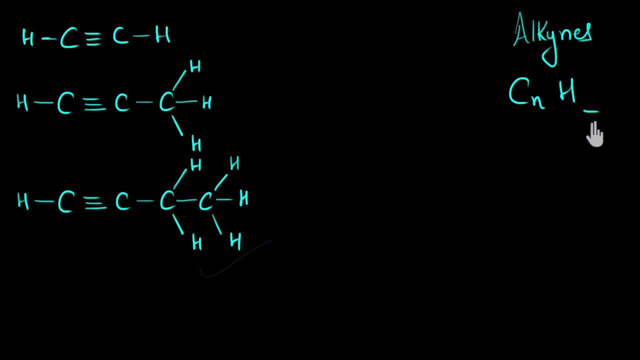 then how many hydrogens will it have? Okay, So try it by yourself first. Now, if you have tried it, let's see So over here. the molecular formula of this compound is C2.. There are two H, there are two carbons and two hydrogens. 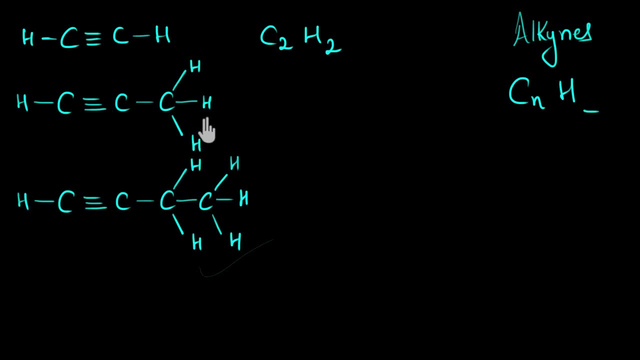 So C2, H2.. The molecular formula of this is three carbons, So C3 and H1234, H4.. This one has four carbons, So C4 and H123456, H6.. Okay, So, if you see in general, 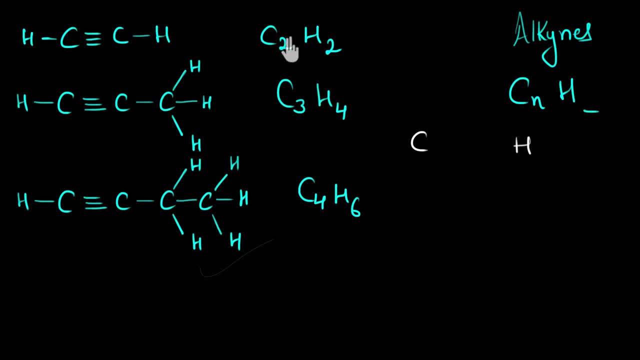 then let me prepare a column over here. C and H, I see. for two carbon, there are two hydrogens. For three carbon, there are four hydrogens. For four carbon, there are six hydrogen atoms. Okay, Now, what's the relationship over here? 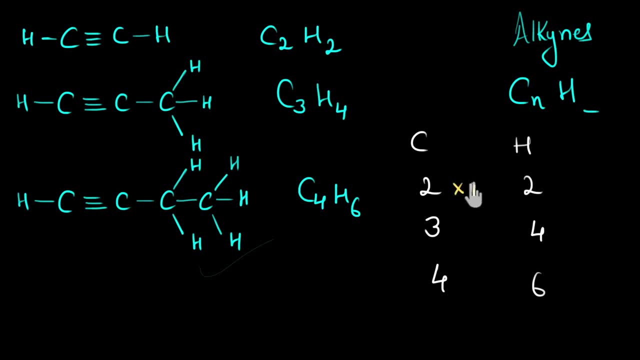 Hmm, Maybe the relationship is two into one. Into one is the relationship. Okay, If I try it over here, then this does not give me the answer. Three into one is not four, but three So multiplied by one is not four. 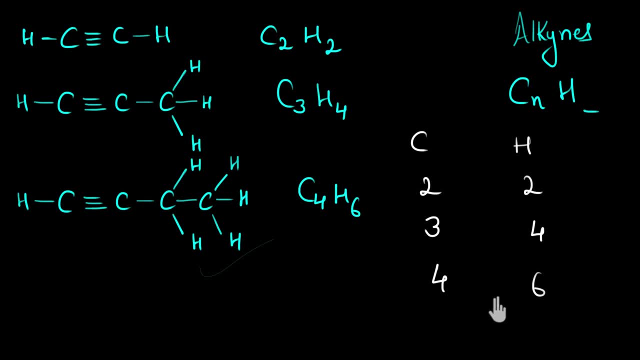 Three times by one is not going to be the answer. What about? okay, over here? if we see, then four plus two is six. So plus two may be the function, Plus two may be the relationship. So but if I do, plus two over here. 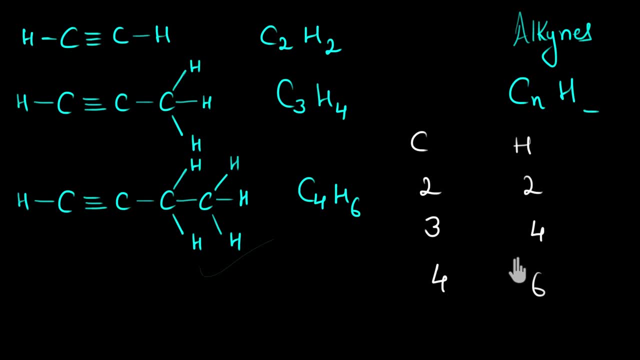 I should get five, not four. So plus two can't be the answer. Hmm, What if I multiply this by two, Four twos are eight, And then eight minus two is six. So into two and minus two. This should be the relation. 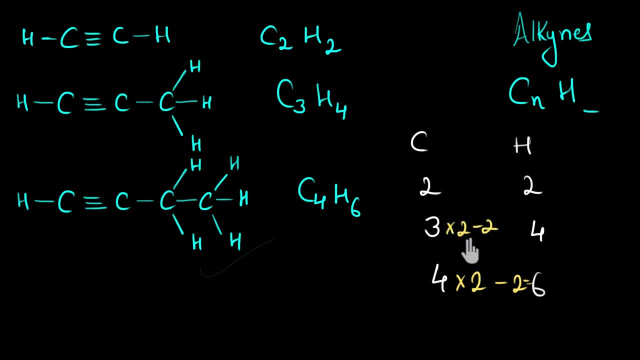 Let's try it Into: two minus two. So three twos are six Minus two is four. Yes, I'm getting it Once again: two into two and minus two. So two twos are four Minus two is two. 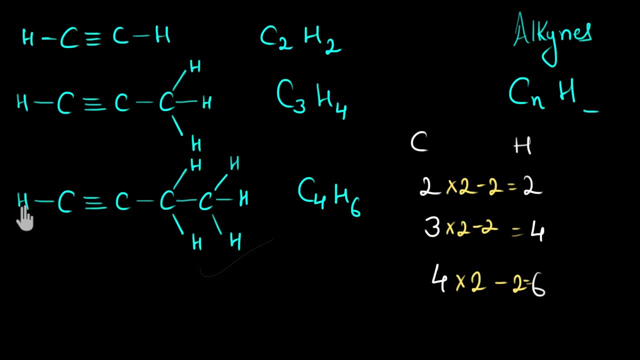 So yes, this is the relationship Into two minus two. That means if you have N carbon in a simple alkyne, then the number of hydrogen atoms will be twice the number of carbon atoms. Two N and minus two. This is going to be the general formula. 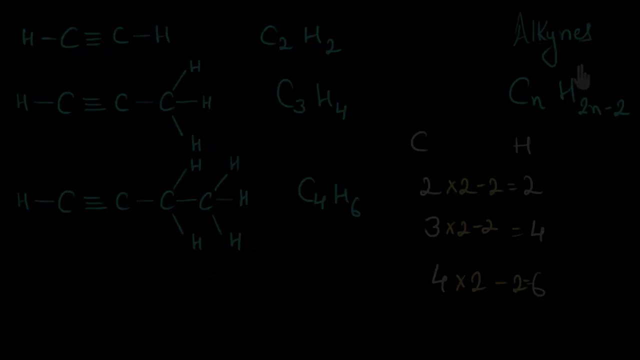 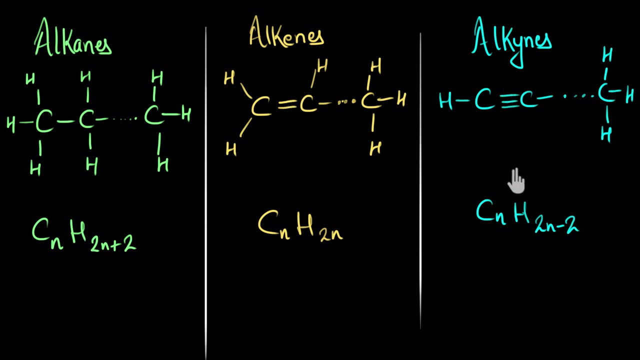 general molecular formula of simple alkynes. So in this video we looked at the members of the alkane family, the simple alkynes and simple alkynes family, And we also looked at their general molecular formulas. Well, if you are very keen, 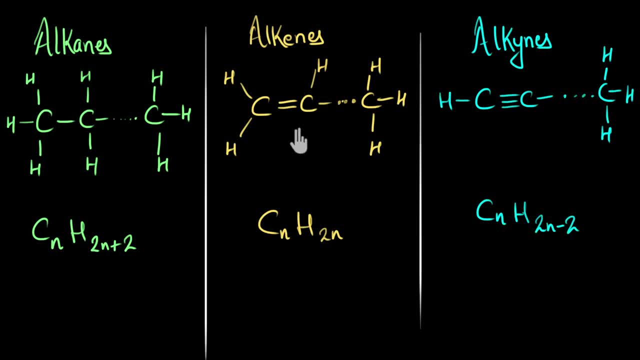 you would notice that the only difference between alkynes and simple alkynes is that there is a double bond And rest of the things are exactly the same. So the difference between their molecular formulas could only be because of this double bond. If I had to put a double bond over here. 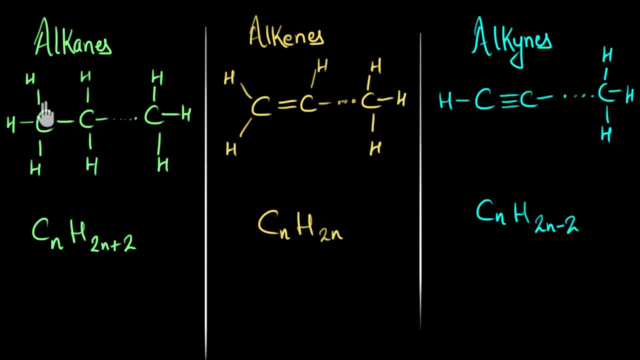 I would need an electron from this column, this carbon and this carbon. So if this carbon lets go of this hydrogen, then it can have an extra electron. Similarly, this carbon can also let go of the hydrogen and get an extra electron. Now these electrons can bond and form a double bond. okay. 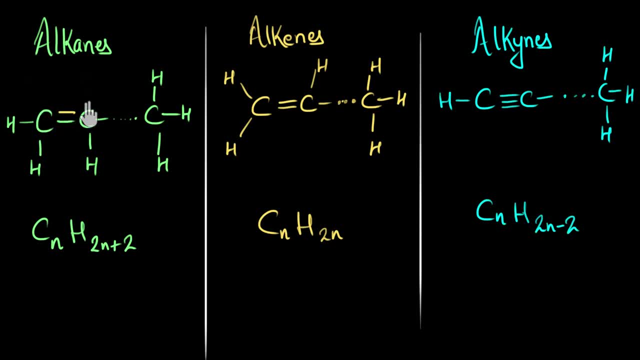 So to get a double bond over here, I had to let go of two hydrogens, And that's the difference between an alkene and alkene. See, this has H2N plus two, whereas this one has H2N- the differences of two hydrogens.